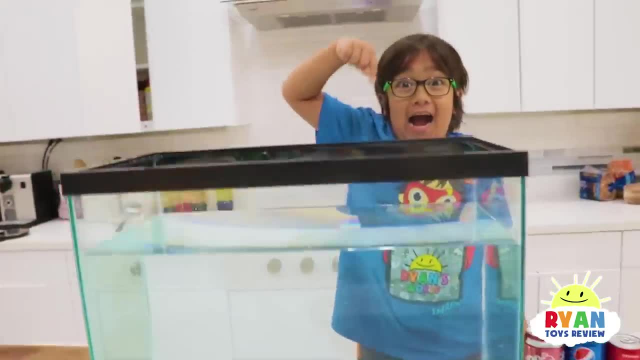 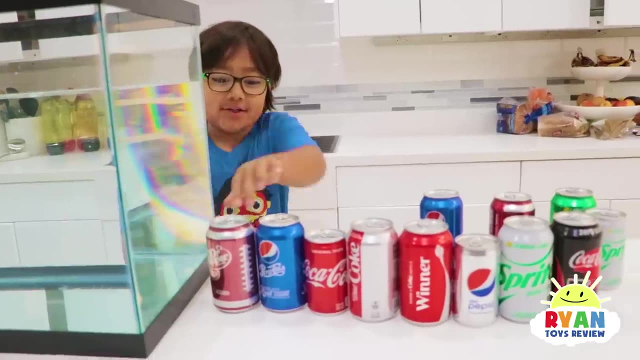 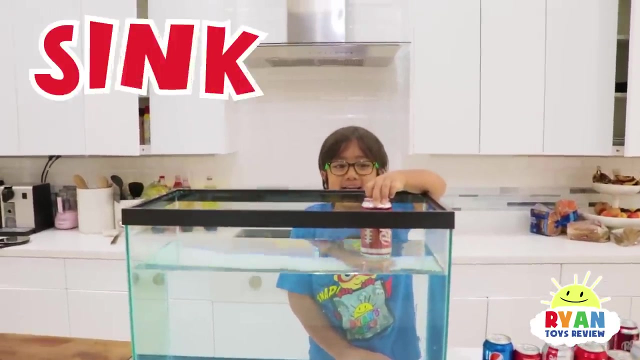 That's right. We're going to drop those soda cans in the fish tank over here filled with water, and we're going to see which one will sink and float and why. First I want to try this one That is Dr Pepper. Okay, let's see Sink or flow. What do you guys think? I think it's going to flow. It's going to sink. It's going to sink, Okay. 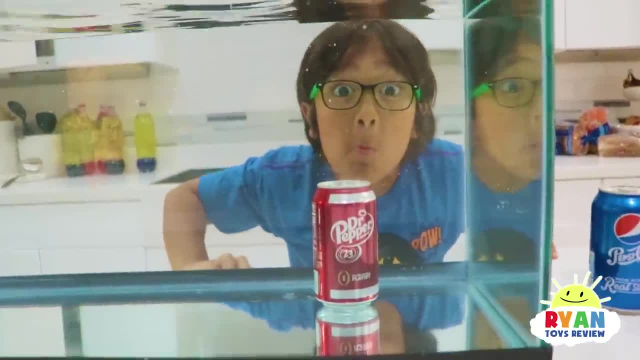 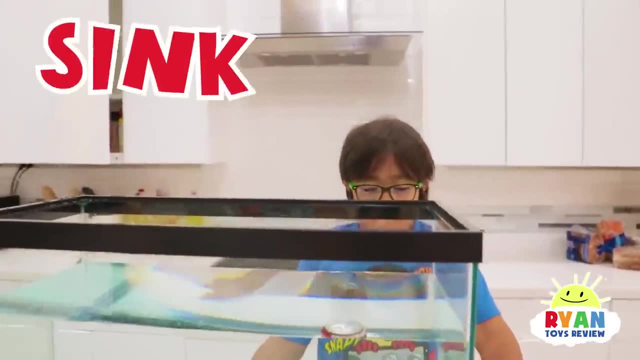 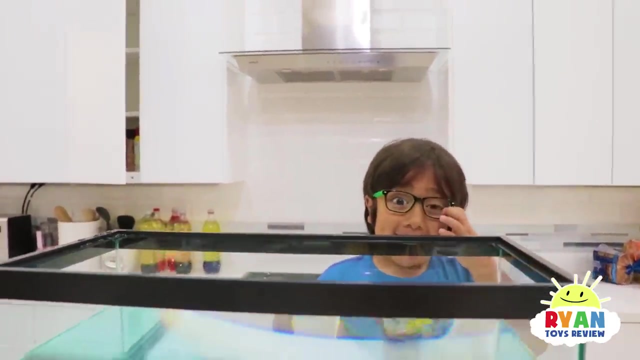 I was right. Yeah, it's sinked all the way down. Whoa, Ryan's in water. Whoa bubbles, Yeah. so why does things sink and why does things float? Ryan knows this. Because the density is too high or too low. That's right. If the density is higher than water, it will sink. 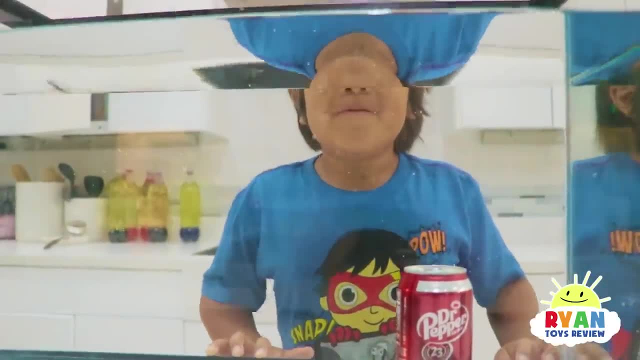 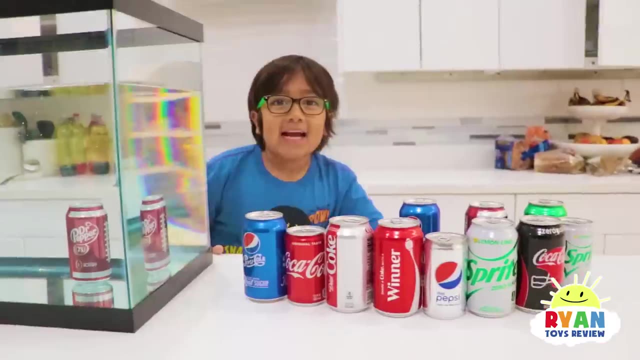 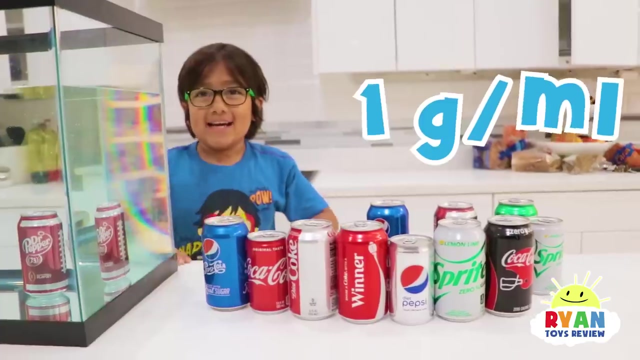 And if the density is lower than water, it will float, And if it's the same density it will hover in the water. Good job, Good observation. And the density of water is one One. what One One? One gram per milliliter. One gram per milliliter. There's other units, but yeah, Okay. 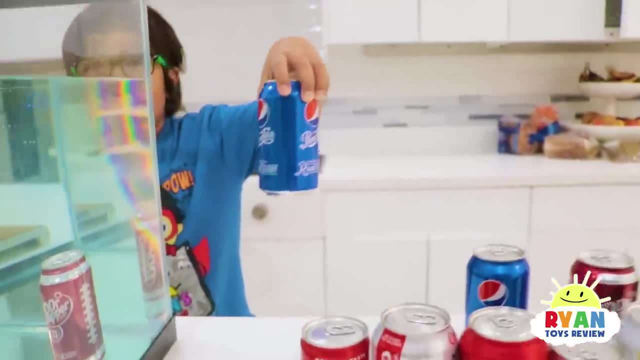 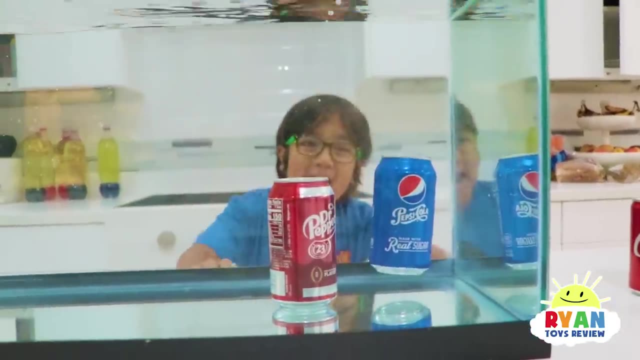 Ryan wants to test out Pepsi, Pepsi, Regular Pepsi. What do you think? I think it's going to sink. It's going to sink. Okay, Let's see I was correct. Wow, they both sink. Whoa, Whoa, It was floating for a little bit. Yeah, it did. You guys see that. 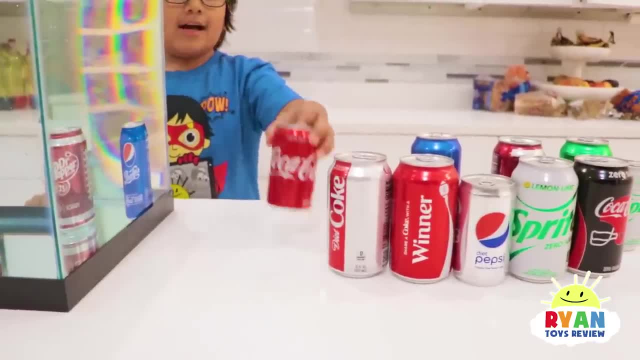 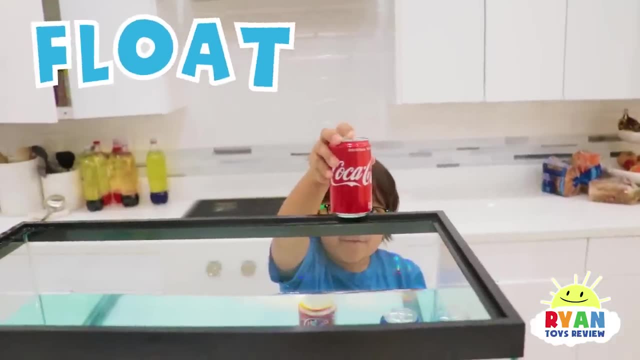 Okay, what else do you want to test out? And then Coca-Cola. Yes, but this bottle is smaller, though, Ryan. the can is smaller. so what do you think if it's smaller? I think it might float, Float. okay, let's see. 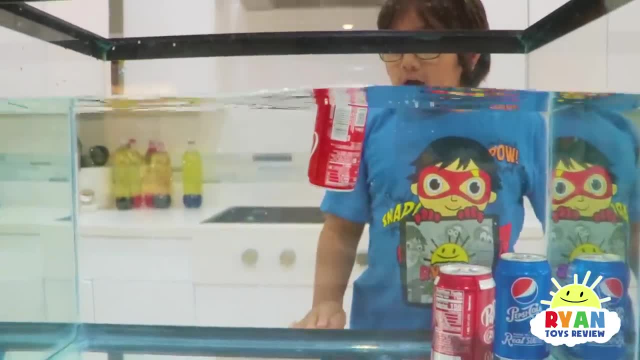 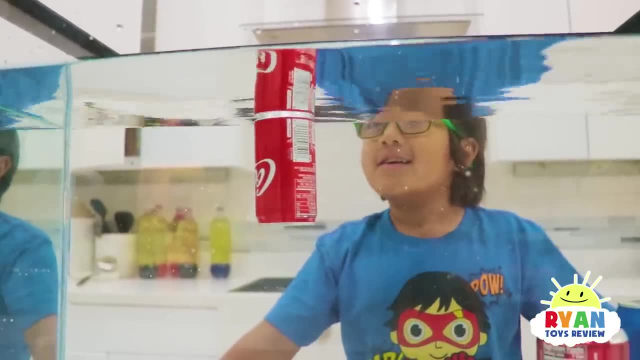 Let me see: Oh, it's gonna float, Oh I love, oh, oh, oh, oh, it floats, It floats. What? Or is it the same density, Maybe what? Come on, we're gonna wait a while. 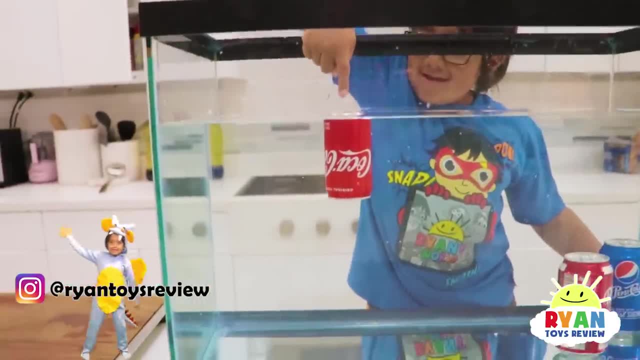 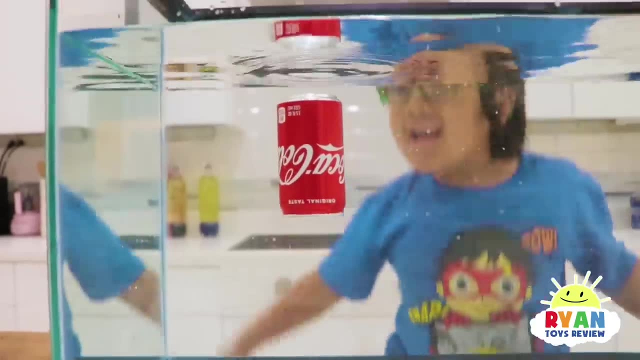 and see what happens to that Coke can. okay, Do all the small bottles float. Let's try to push it down. let's see what happens. Let's see What It just goes back. it just hovers on there, wow. 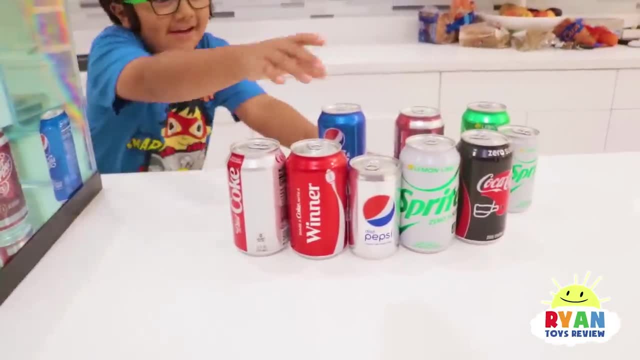 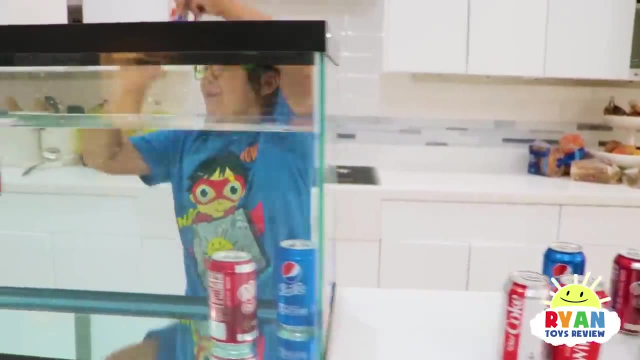 Okay, let's try a smaller bottle too. Let's see what makes a difference. Oh, okay, let's do this one, But that's Diet Pepsi. Do you think Diet and regular have a difference, though? No, Let's see. 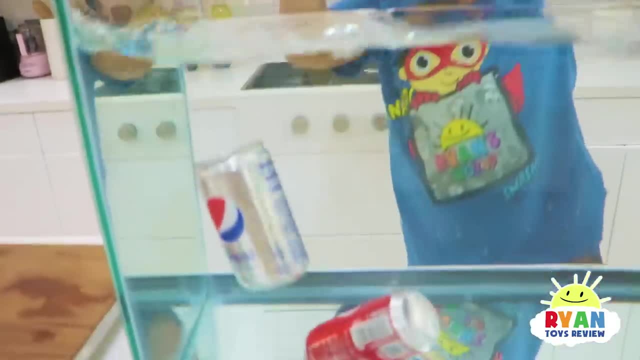 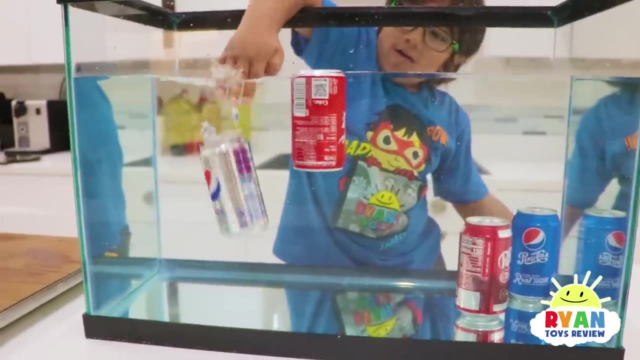 Wait, what if we put it on top? It's probably gonna fall off, though. What they both float. Oh, wow, Oh, this one floats a little bit more. Oh, it's like I'm gonna go back up interesting. 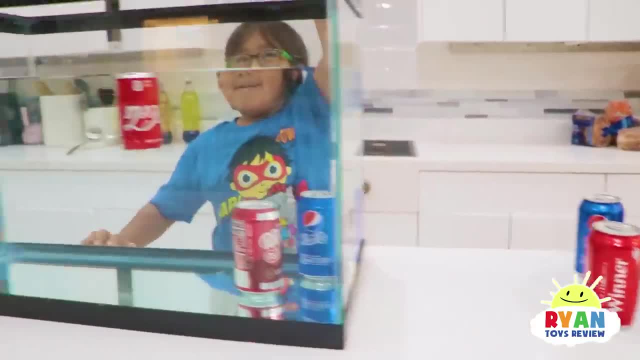 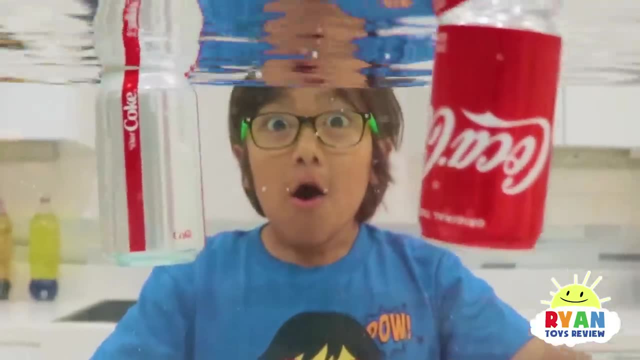 Whoa Coke. I don't think it's gonna float The Diet Coke. That's Diet Coke, Let's see. Wait, what, What, What. but that's a big can too, Ryan, why does it float? 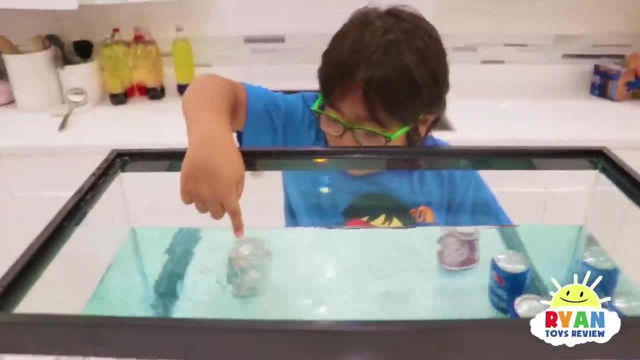 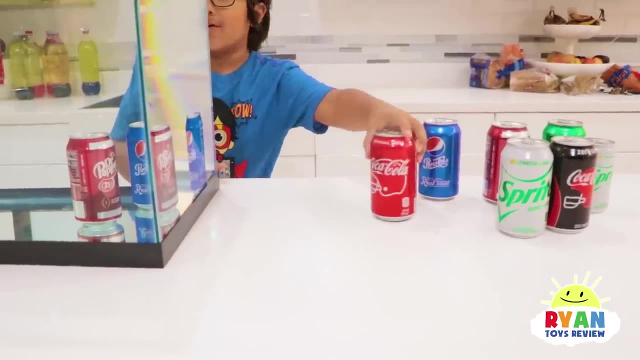 Huh, we gotta put more and see What What is going on. And this is Coca-Cola, the big version, That's right. so the small version, float. what about the big version? Wait, let me see how heavy this is. 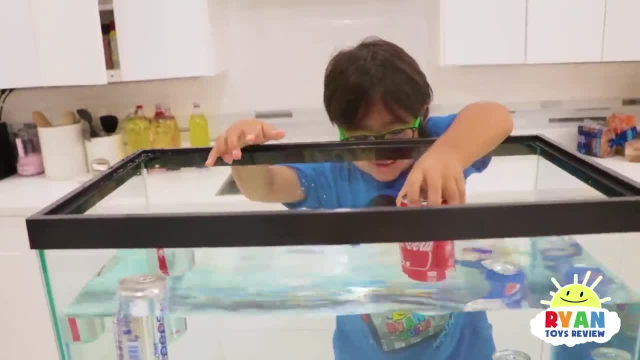 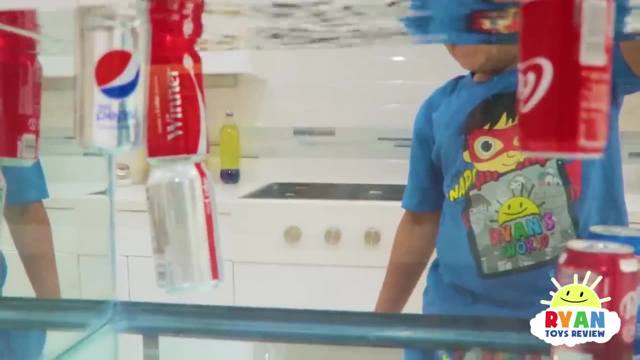 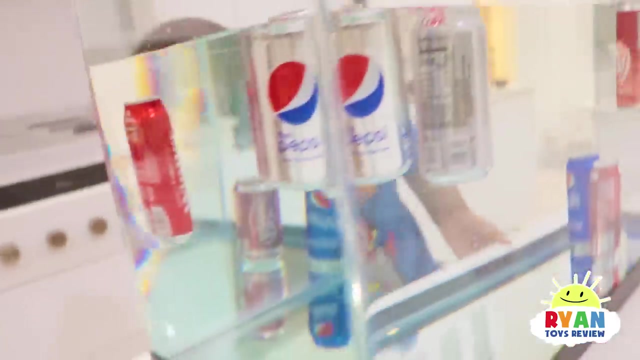 Oh, this is way heavier. I think it's gonna sink. Look at that, Whoa, What, How, What is going on That Coke? there is still wait, stinky, It's still wait, stinky, It's still wait, stinky. 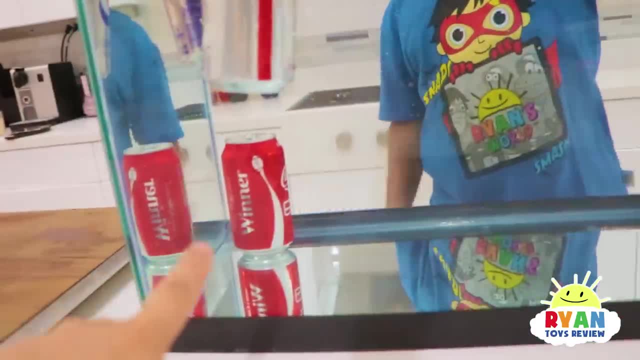 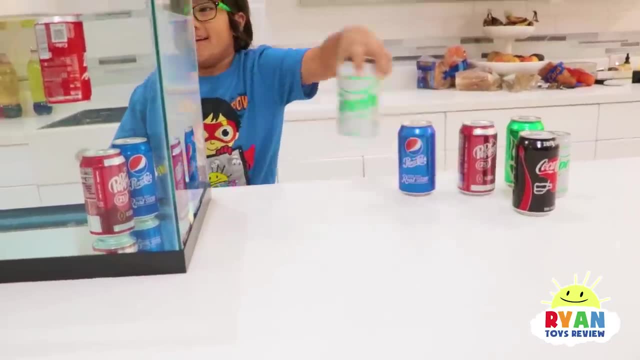 It's still wait, stinky. The small can float, but the big can sink, but then that's a big can, but it still floats, so Interesting. okay, Let's do Sprite. That's a Diet Sprite. so what do you think, Ryan? 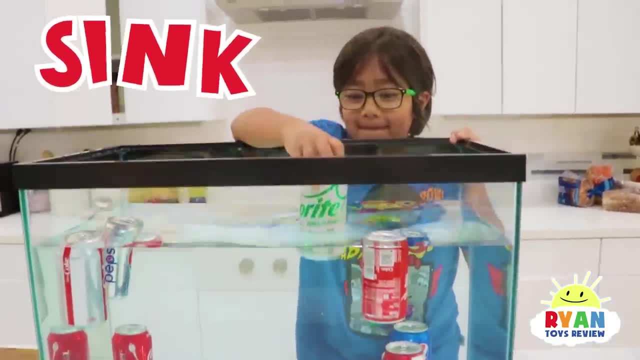 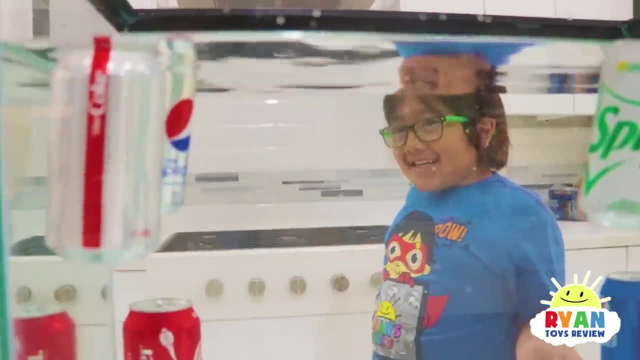 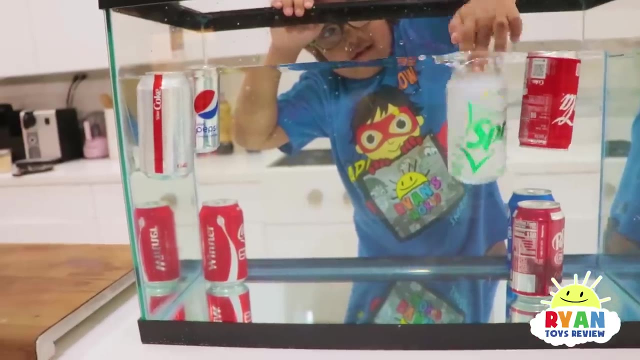 Is the no sugar gonna float or sink? It'll sink, It'll sink. Okay, What is happening? Oh, interesting, right. So both the Diet giant-sized float, Let me see, Let me see, Push it down, Push it down. 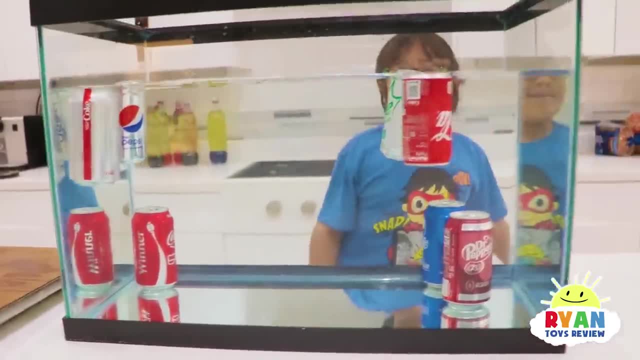 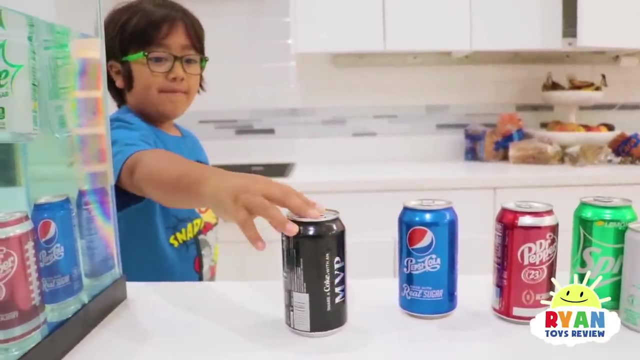 Oh, it actually goes back up. Now let's do MVP. So this is Coke Zero, That's right. So this is also Coca-Cola, but it's zero, so it doesn't have sugar in there. It's different type of chemical. 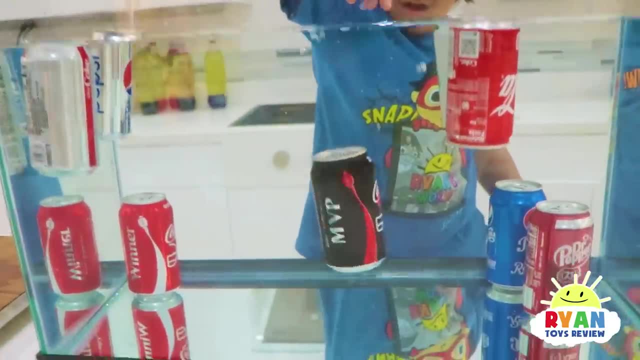 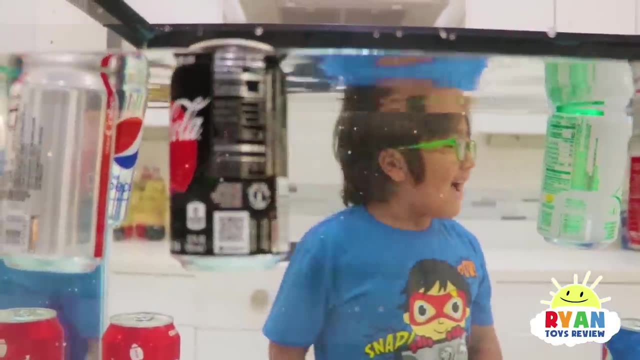 It's gonna float. Different type of sweetener. Yeah, Sweeter, It floats too. What is going on, Ryan? It flies, Huh, And these have you already. Oh, there's a smaller one. Okay, smaller Sprite. 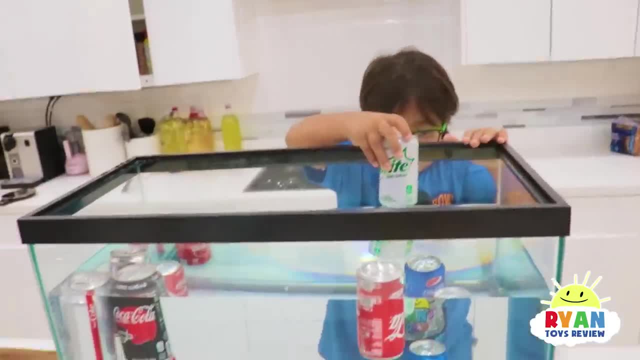 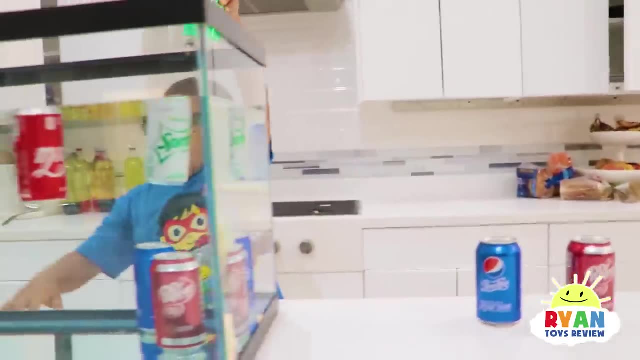 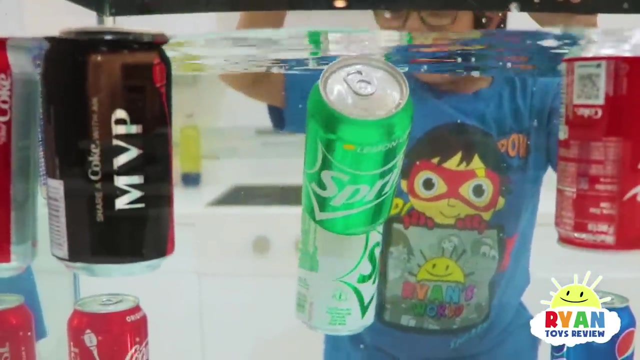 Let's see, That's also no sugar. Ryan's smelling it. We never tried this one yet That's sugar. Okay, that's a regular Sprite and it has sugar. Oh, Take that. I think it's going to float. 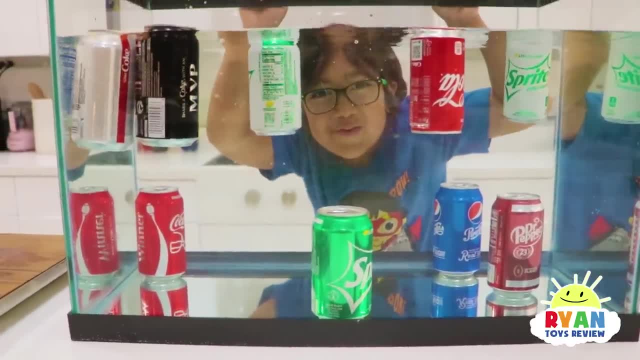 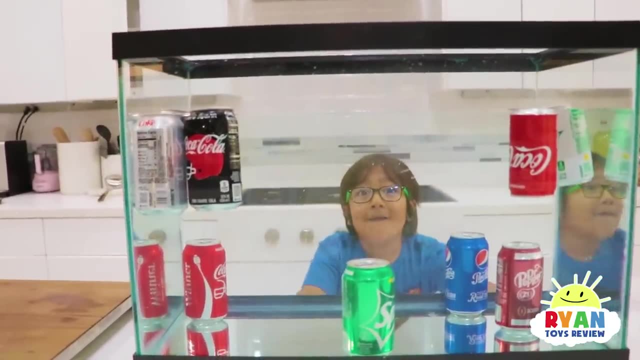 Yup, Wait, wait, wait, Ha ha ha ha. It sank Whoa, Whoa. What did you observe with all these soda cans? All the diet ones? float, That's right, Except for this one. That's not diet, but it's float. 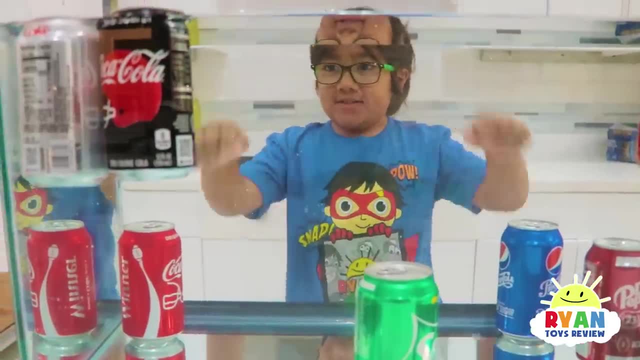 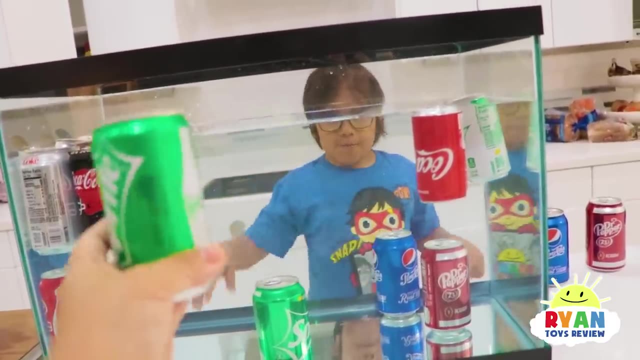 And what happened to all the regular sodas? They all sink. They all sink, Yeah, except for this one. So I actually found another can here. It's a small version, It's regular, so we're gonna test it out and see. 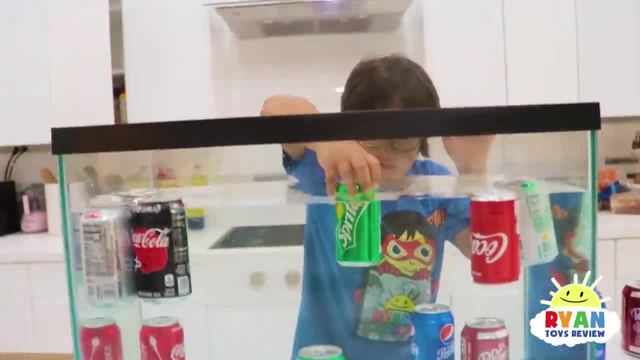 Do you think it's gonna float or sink? Oh, it's so cold. Yeah, it was in the fridge, so It's gonna float. It's gonna float. Okay, let's see, Let's see, Let's see. 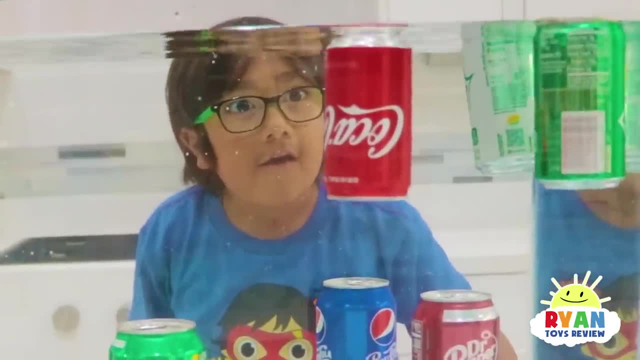 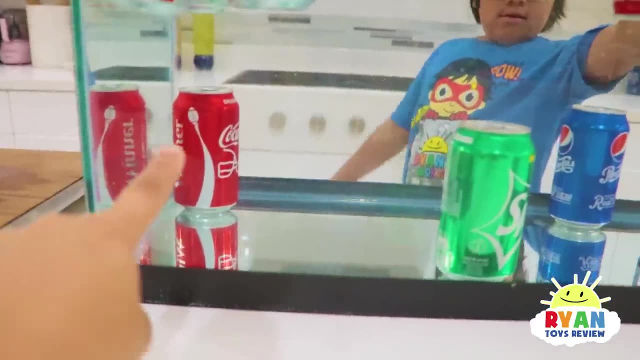 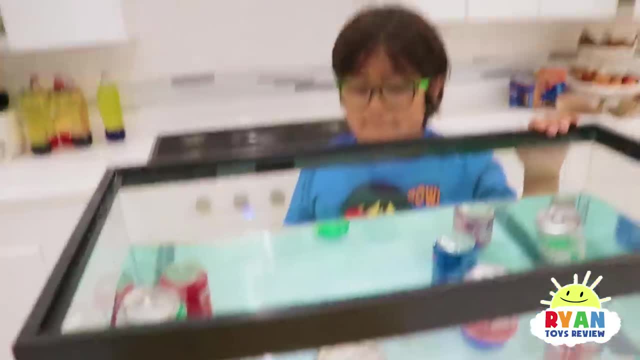 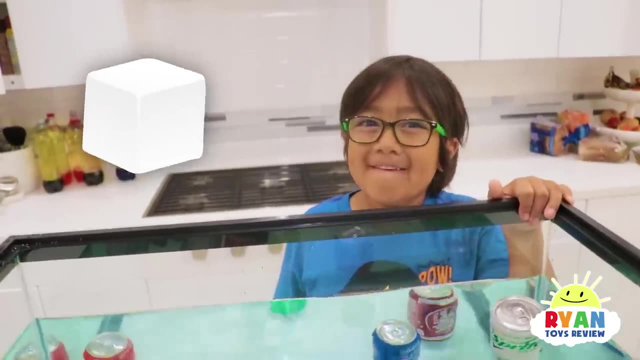 but if it is diet, it floats, right. Yeah, Do you know why? the diet one floats, but then the regular ones sink all the way to the bottom Sugar, The sugar Good job. So I think these float is because they're smaller cans. 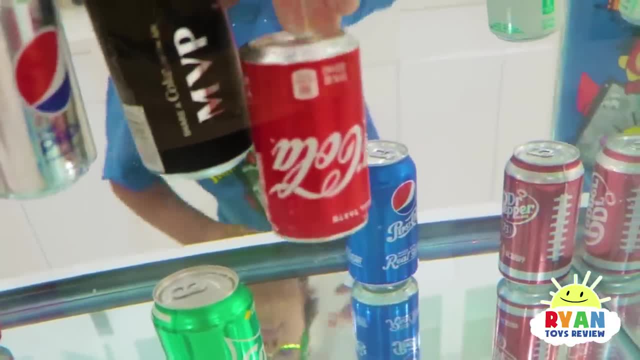 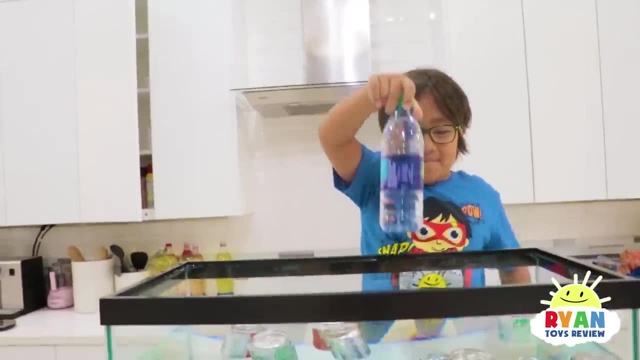 I still know that one's gonna sink. So it doesn't have as much sugar, so it'll still float. See, Yeah, that's so cool. Ryan wants to try a regular water bottle. Let's see what happens. I think it's gonna sink. 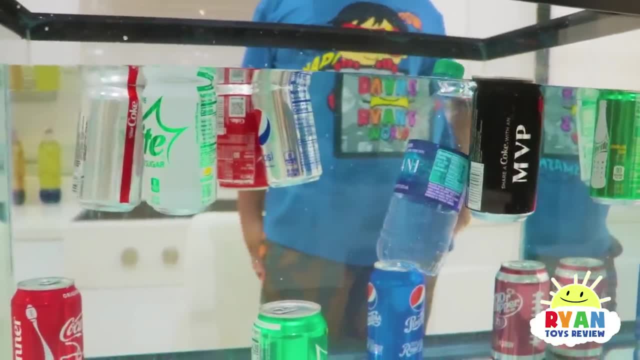 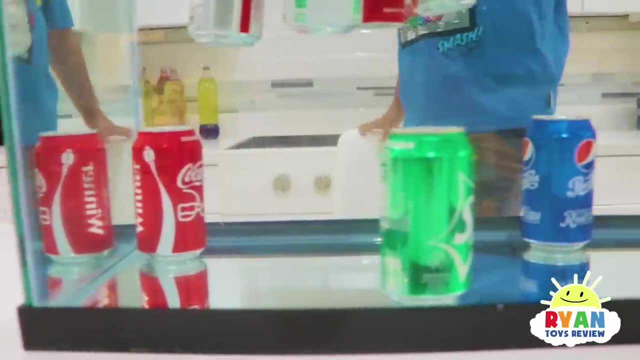 Sink. We know it's gonna float. Whoa, Whoa, it's hovering. Maybe it's the same density because there's water inside. That's right same density as water. So all the one with sugar is sinking on the bottom. 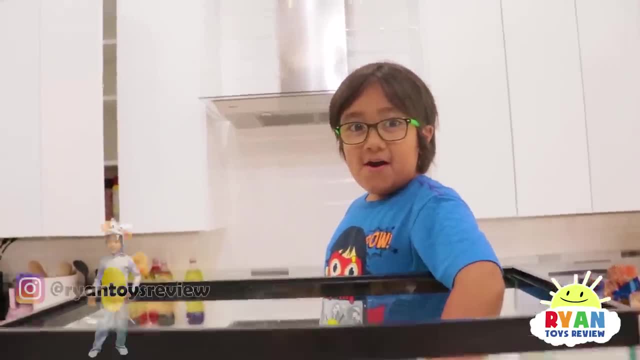 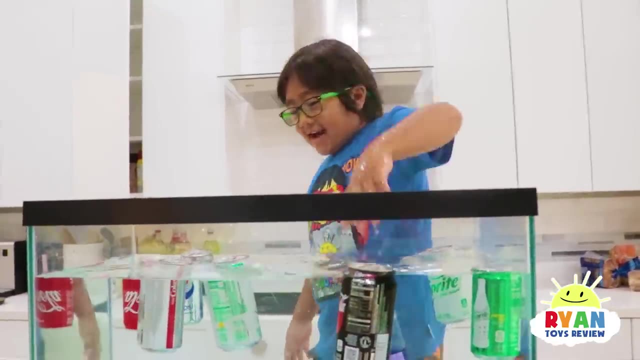 Do you know how much sugar are in sodas? Uh, no, A lot. But before we get to that, let's test out other items around the house. Let's go, Okay, let's go. So we're gonna go and get some items around the house. 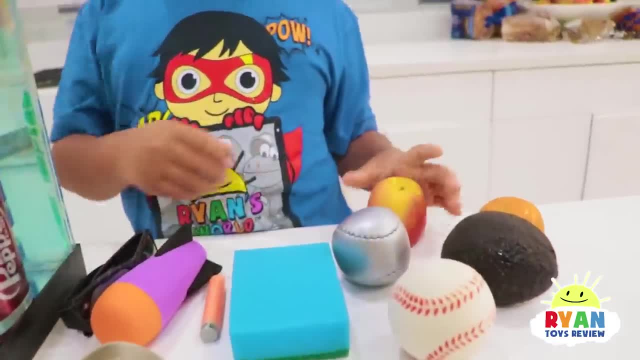 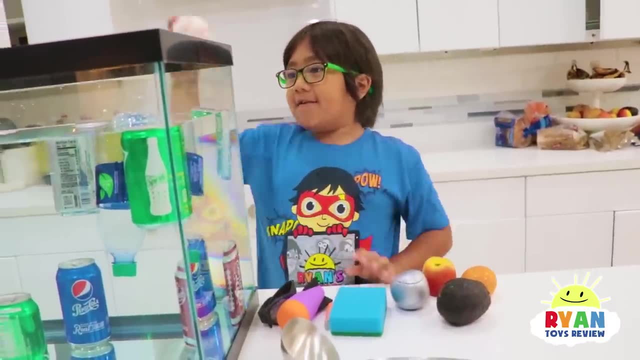 and test them out. Now we're gathering stuff around the house and these are real, Okay. so which items do you wanna try first? I'm gonna try the baseball. Ooh, okay. So it's a squishy toy. it's not a real baseball. 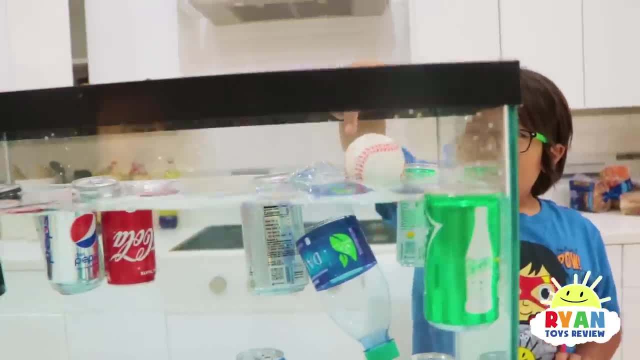 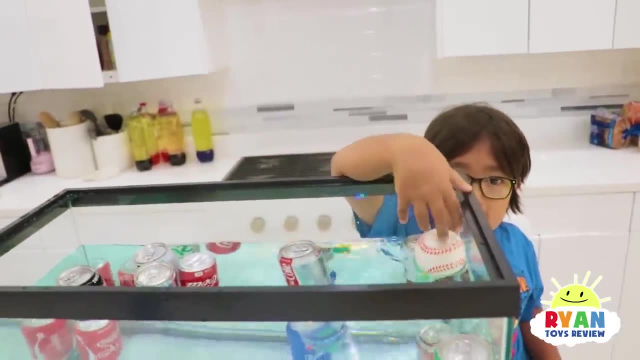 It's gonna float. It's gonna float, Whoa, Whoa. definitely float here. Whoa, I didn't know that. I didn't know that. I didn't know that this was less density. Yeah, it is less dense than water. 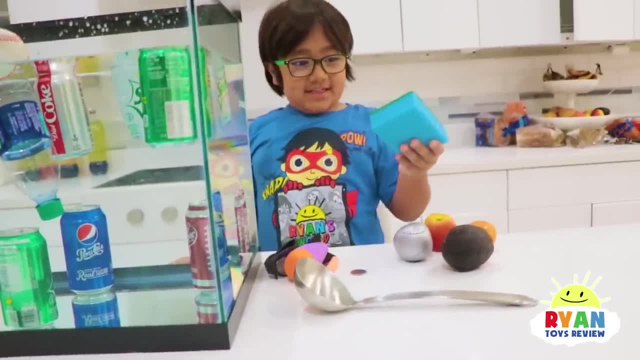 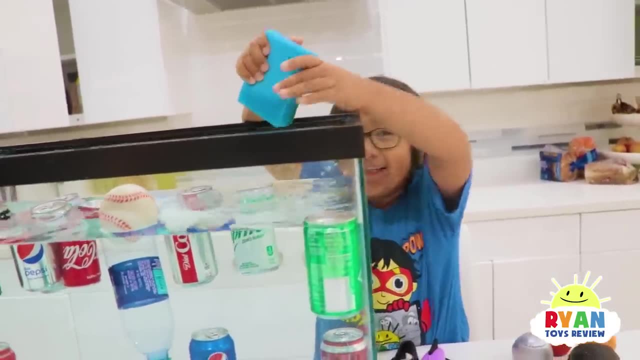 That's why it's like staying on top. What else This? A sponge, It's a sponge, Secret float. Let's get it, Let's get all that. Wait, doesn't this make it like heavier? Yeah, Float. 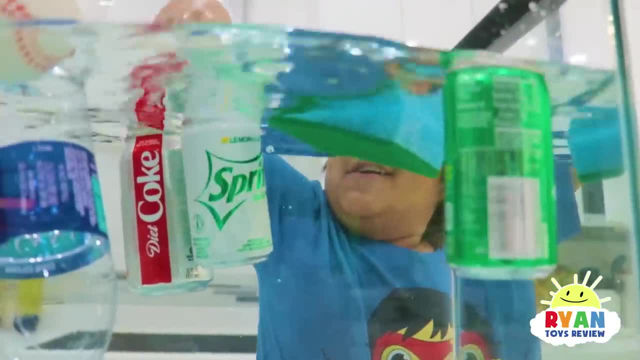 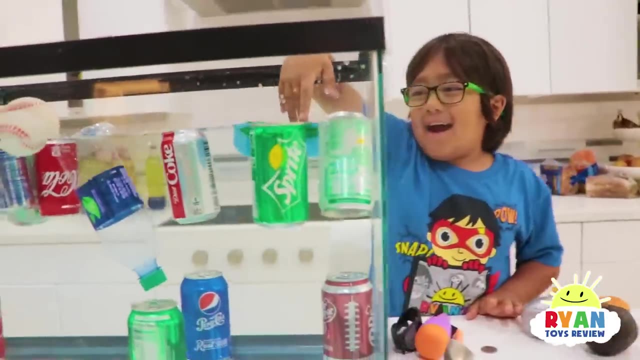 Wait. so if we put water in, it Still float. Nope, still float. Ryan's trying to push it down. Oh, wow, Whoa, Still float. Wow, Looks like you're not getting me down, Ryan. We can try this. 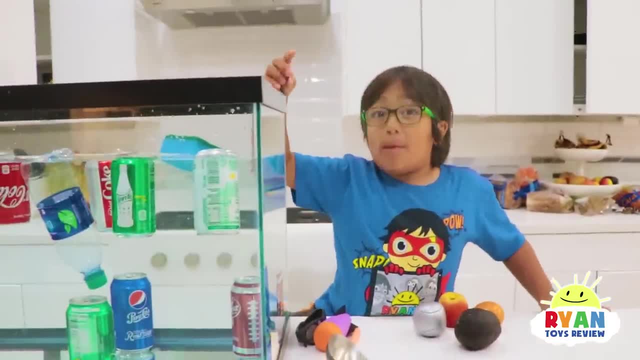 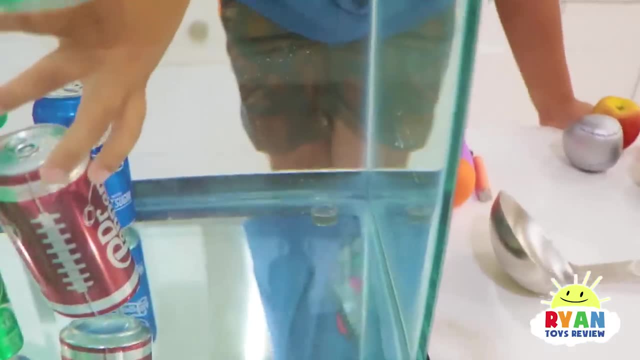 Okay, so we have a quarter, Yeah, but it's gonna be probably a different result with the penny and stuff. maybe I don't know. Oh, It just went all the way down. Where'd it go? Oh, there it is. 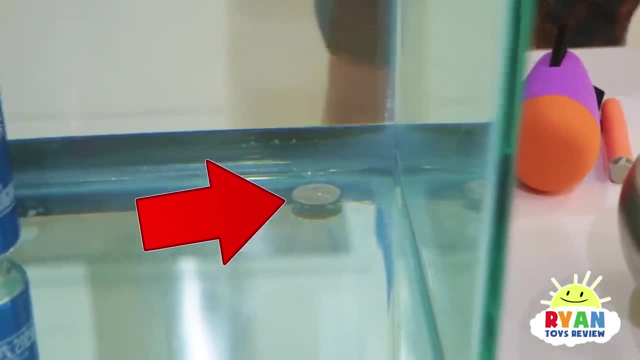 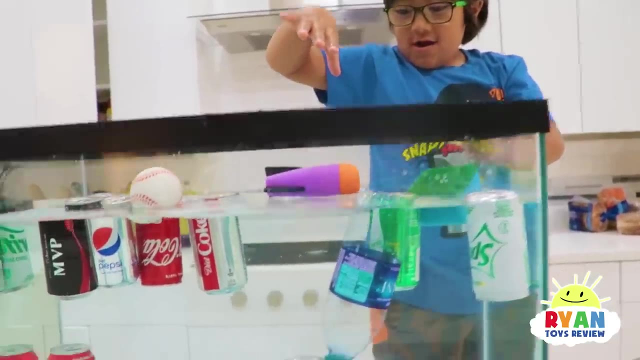 You guys see it, It's right there. So it's sinked. Definitely way more dense than water. Yep, and now we got this Nerf bullet. Let's see: Sink or float. Whoa, it's like a sponge, huh. 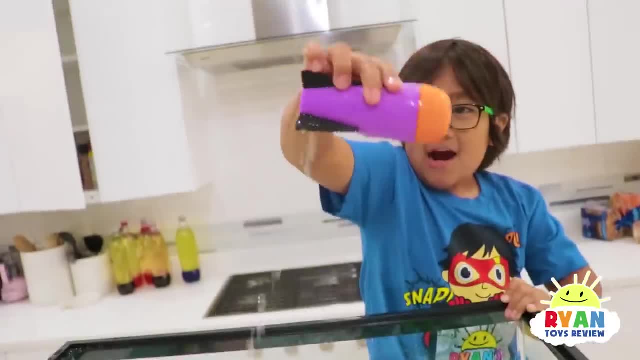 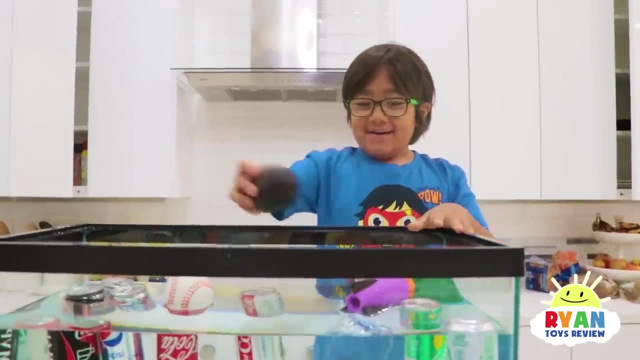 It just like stays on top, On top. Whoa, That's cool. And now we can try this Avocado Real, Real avocado Sink or float, you guys. Oh, it's going up, Ryan, It's going up. 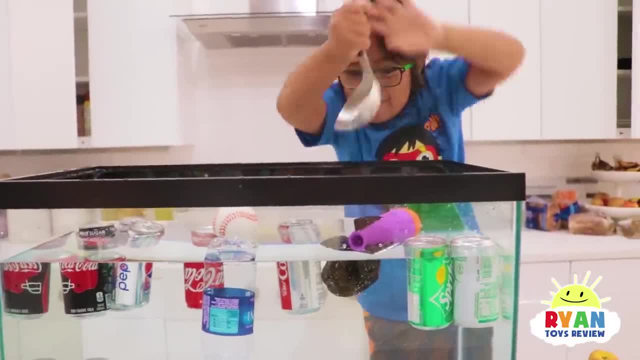 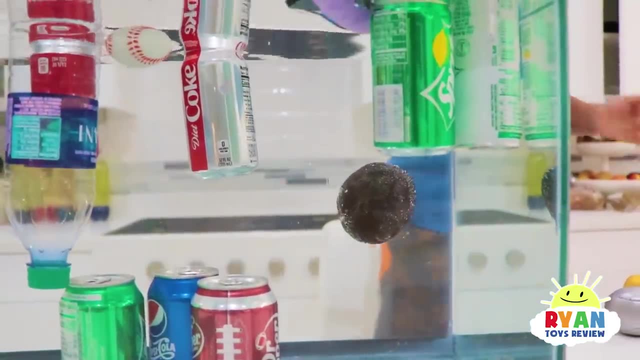 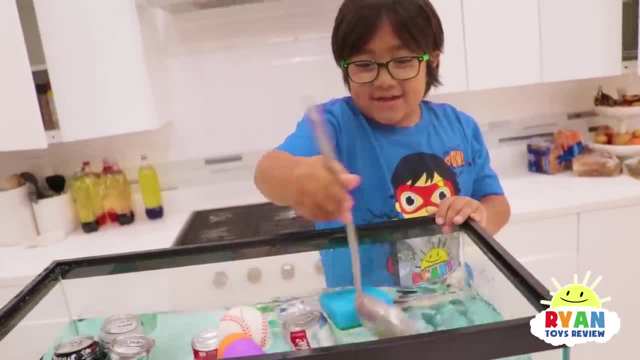 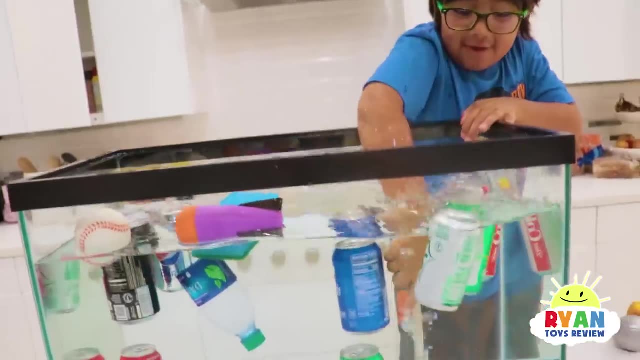 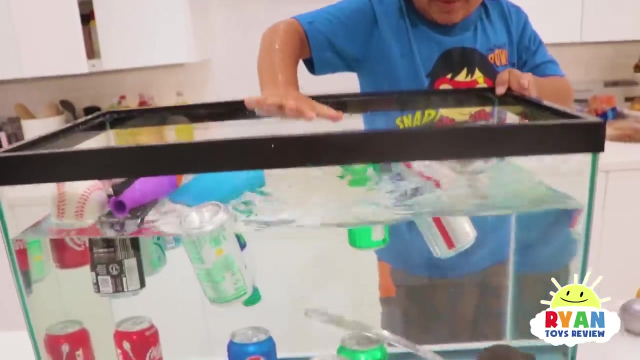 I got an idea, So we can put this in: Uh-huh, Oh, That's definitely sinked, Got it. Now what if I scoop, scoop the avocado up and then drop it? Oh, oh, I have an idea. 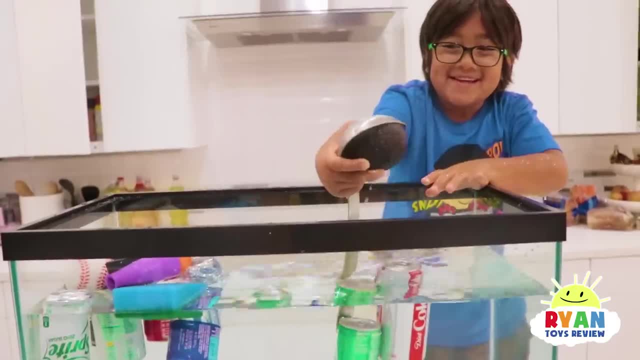 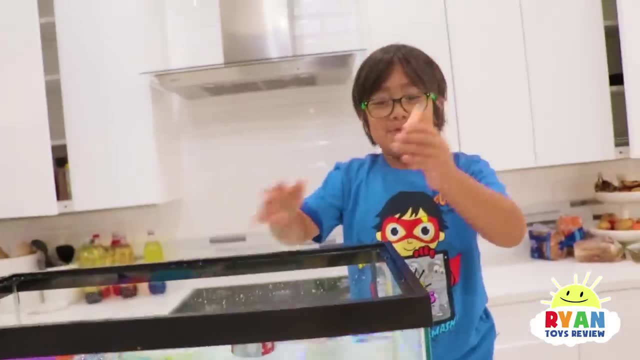 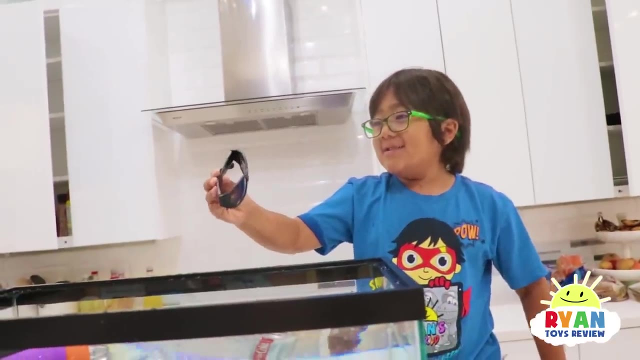 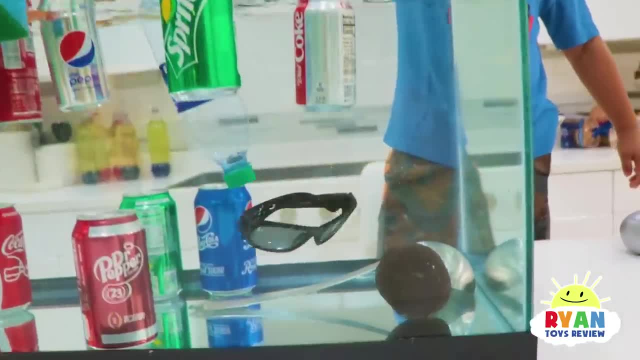 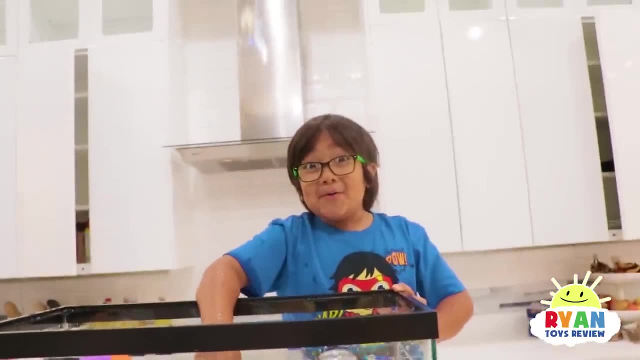 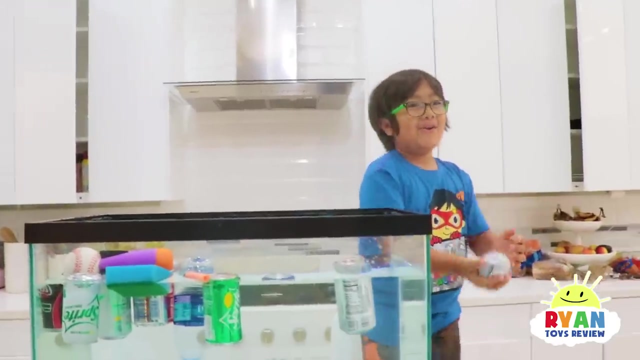 Yay, Bye-bye. So there you go. If you ever drop your glasses in the pool, it's going all the way down, So make it water protection. Yeah, Now we can try baseball. Juggling ball, Juggling ball. 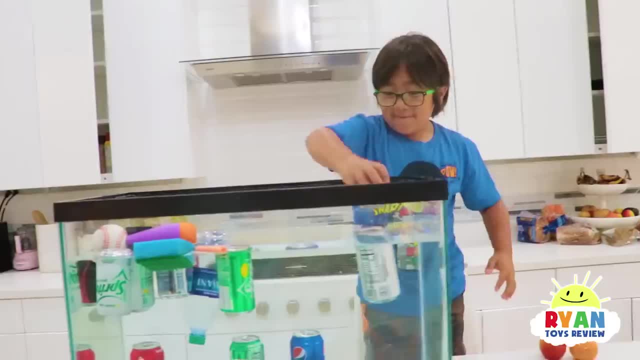 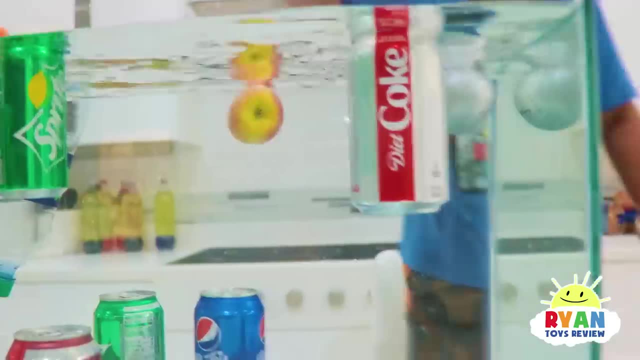 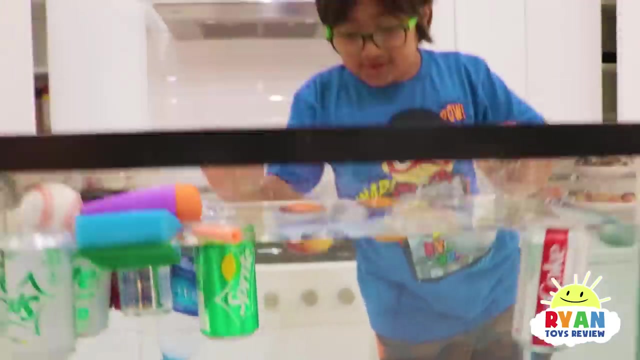 Yeah, There you go, It's going to float. Yeah Yeah, Apple is floating too, Wow, Orange, Wow, Wow. They all float. All the fruit so far that we have in here floats. So far, most of it floats. 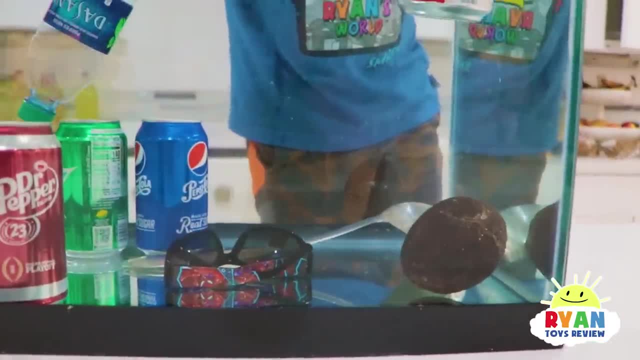 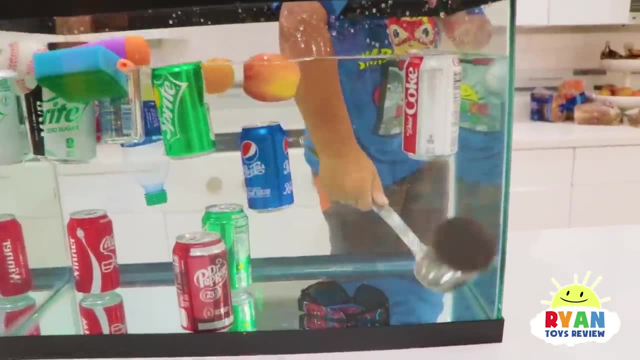 Yeah, Look at that. Oh, except, this avocado is staying down this time. What, what, what, what, Wow, Look at that. No way, Wow, Is there too much water inside or something? Maybe I don't know. 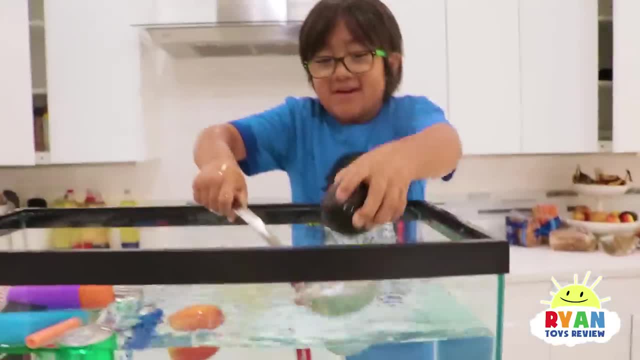 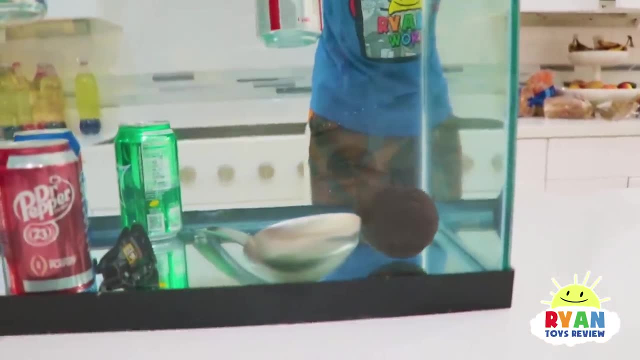 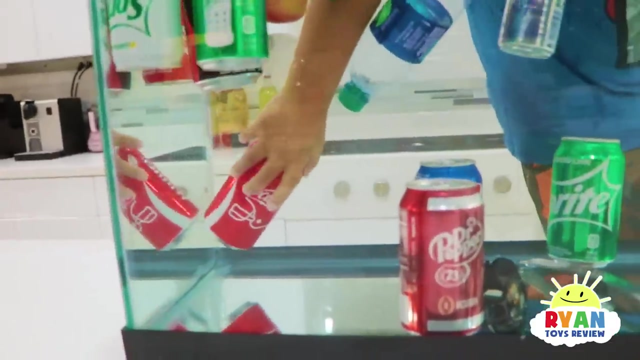 What Well it's sinking now. Oh, let me see Ryan's trying to dry it off. What? Maybe the water got inside and lay it down? Yeah, All the Cokes that sink. we notice that they're regular Cokes. 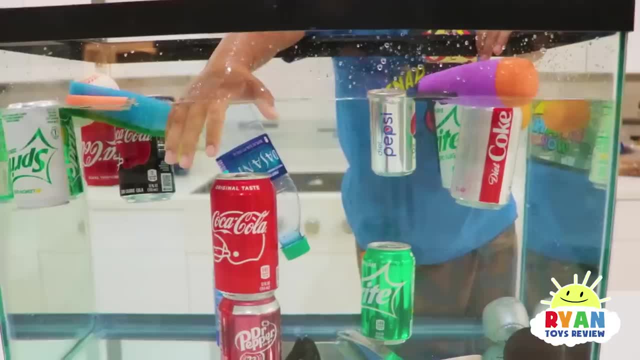 with a whole bunch of sugar inside, right, Yeah, So Ryan's going to pick up the Coca-Cola- Uh-huh, Uh-huh, Uh-huh. So we're going to figure out just how much sugar is inside, Yeah. 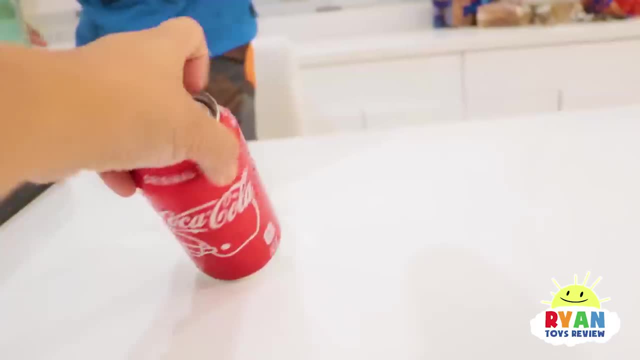 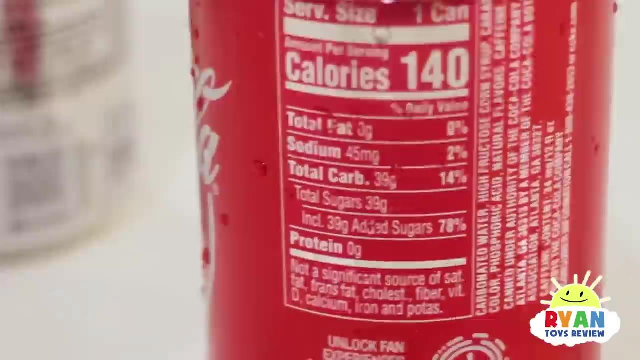 OK. So each Coca-Cola bottle on the back will have a label, And you notice here it tells you exactly how much sugar is inside. It'll tell you It says total sugar: 39 grams. And then here is a Diet Coke. 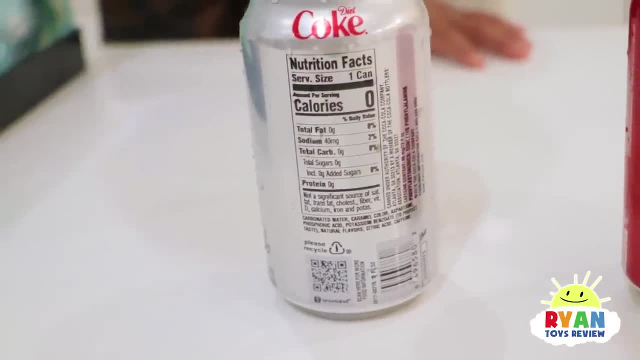 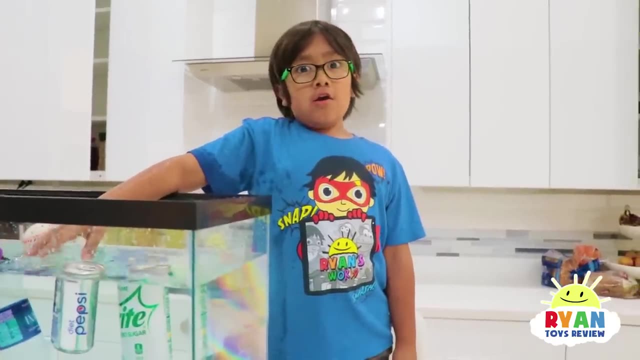 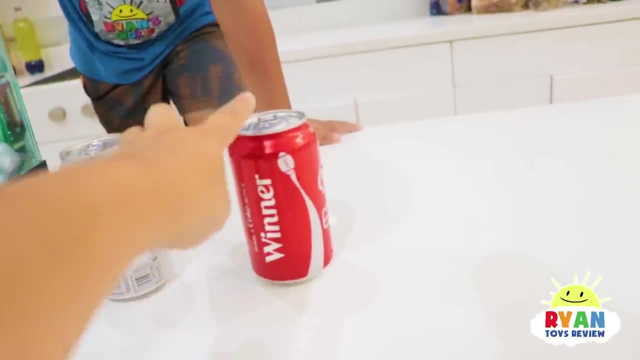 And if you notice here, the total sugar actually says zero. But because there's no sugar, they actually added other chemicals in there to make it taste the same. So it's actually not good for you either, But we're going to see how much sugar is inside this Coke. 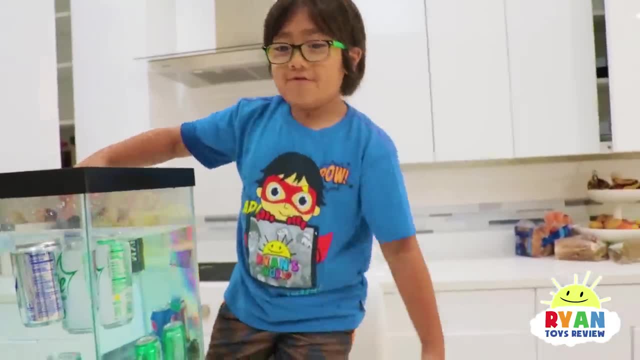 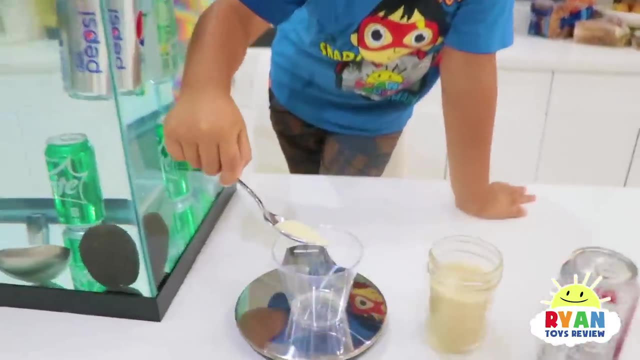 So this Coke? it says it has 39 grams of sugar, right, Uh-huh? OK, I'm going to cup on here. I'm going to zero it out. Ryan's going to put lots of grams Sugar in there to reach 39 grams.